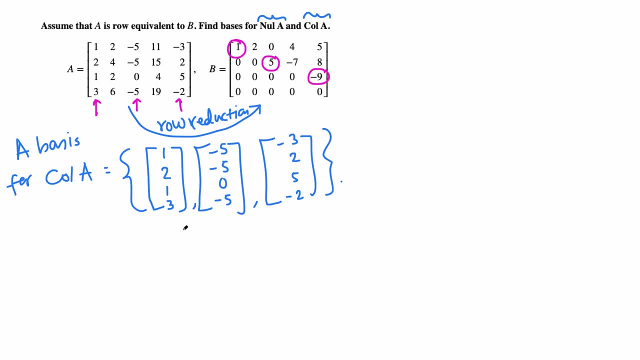 negative 2. easy Now to find the, to find a basis for null a. so null a means we need to solve this problem. So let us solve this problem, get rid of the problem and get rid of the problem. So let us solve this problem, get rid of the problem and. 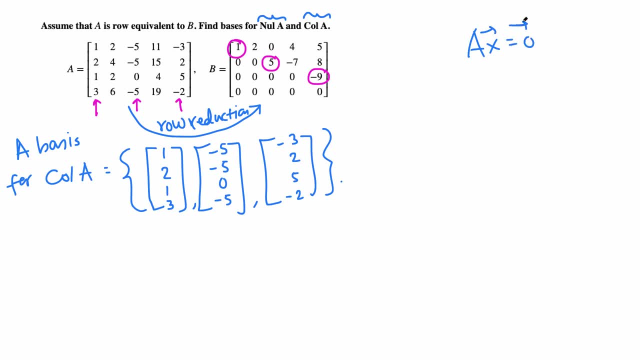 solve this equation: A x equals 0. okay, in fact we can use B, because after we row reduce A, we're gonna get B. so that is same. is this one? okay? so let's do it so B x equals 0. so from here we have now c1. let's say c1, c2, c3, c4, c5, or you can. 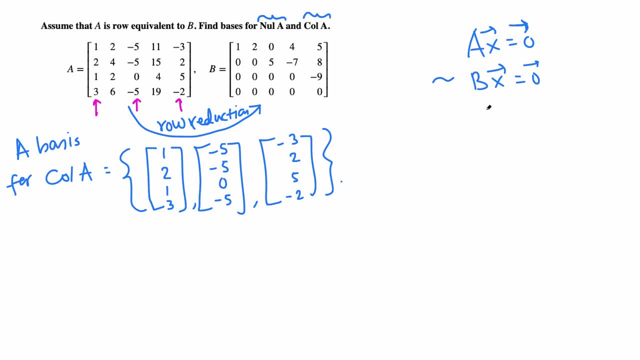 say x1, x2, x3, x4 and x5. so when we solve this, where x is x1, x2, x3, x4, x5, from the last row, there is nothing here. so we got pivot here here and here. so second variable is free. 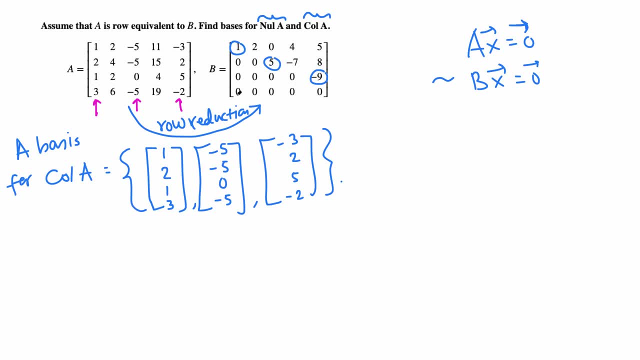 and fourth variable is free, so this one is nothing okay. and from here 9, negative 9. so we get negative 9. so we are saying I'm saying this is x1, x2, x3, x4, this is x5, so negative 9, x5 is just. 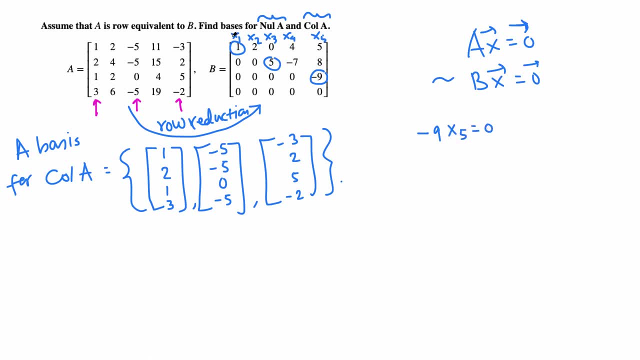 x1, x2, x3, x4. this is x5, so negative 9. x5 is just 0. so this x is in fact x1, x2, x3, x4, x5. okay, negative 9. x5 is zero. that means divide by negative 9, so x5, 0. okay, so we. 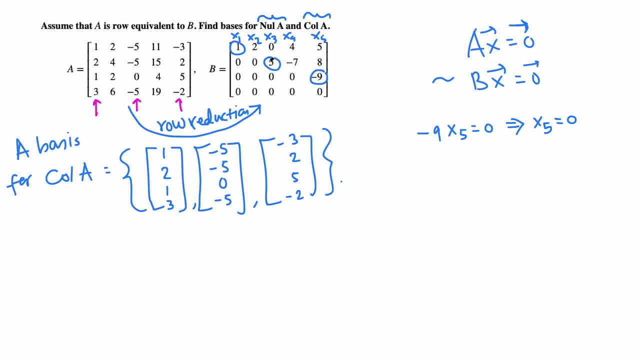 got now from the second row: 5x3 minus 7, x4 plus 8x5 is zero. ok. x4 and 90 are actually zero, but contributes x5.. Now on 7x5.. is 0 and x4 is free. okay, so we got x4 free and x2. those are free variables, so 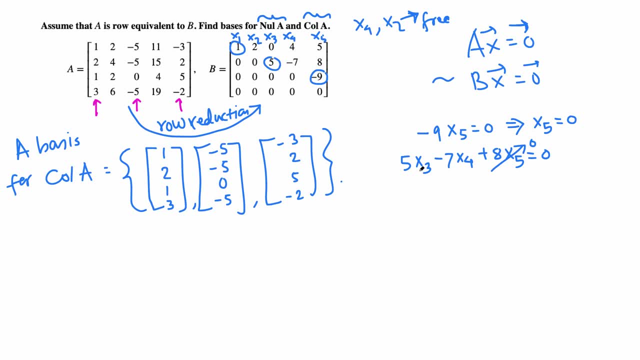 x5 is 0, so this is just 0, so x3 is then what? move this over 7x4 over 5? so 7 over 5x4, where x4 is free. that's from second row, from the first row, we're. 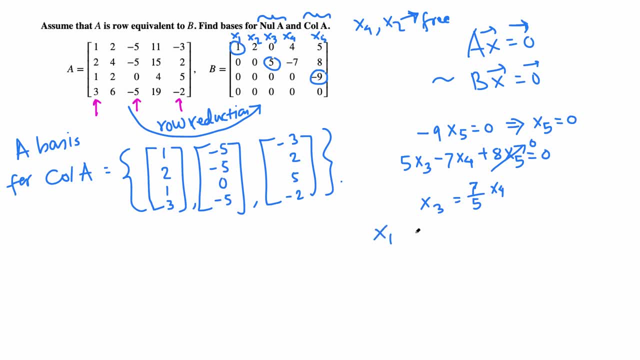 going to get now 1x1, so x1 plus 2x2 and 0x3, not needed- plus 4x4 plus 5x5, so x4, this is. x4 equals 0. But x4 is 0, so this is 0, x4 is free variable and so is x2, so from here x1 is. 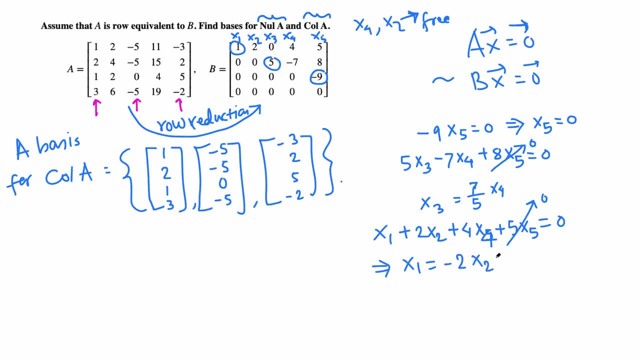 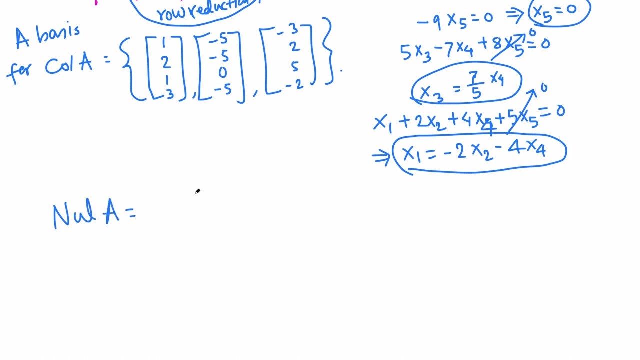 move these two terms over. so negative 2x2 minus 4x4. okay, so we got x5, 0,. x3 is this because x4 is free variable, x2 is also free variable and here is x1.. So we are trying to find a basis for null a, so null a is, in fact, span of this. 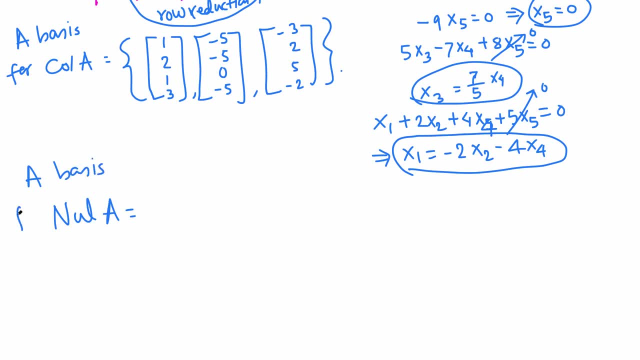 so a basis for null a is just x1, x2, x3, x4, x5, which is we got. x1 is negative, 2x2 minus 4x4,. x2 is free, just x2, x3 is 7 fifths x4, x4 is just x4. 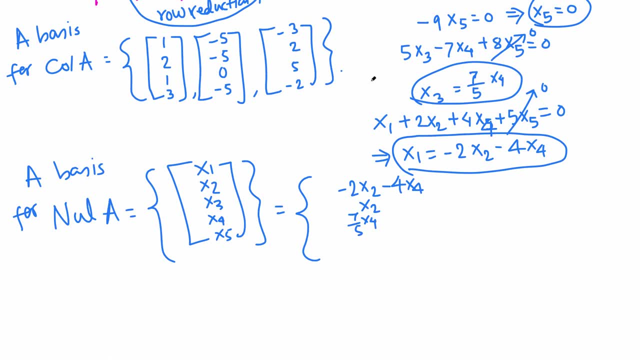 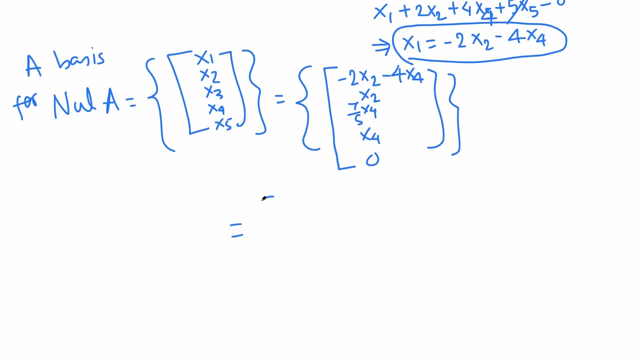 okay: x1, x2, x3, x4 and x5. we found 0.. Okay, so we got two free variables here. we can write in this way: we can factor x2 out and take that away. so that would be: x2 means negative, 2, 1,. 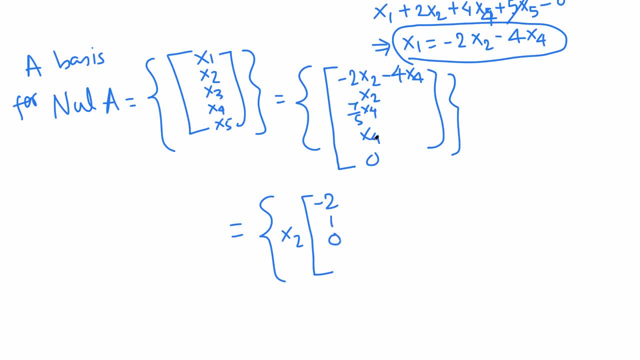 in the second. there is no x2, so 0, there is no x2, 0, 0.. Okay, and from here we can factor x4 out. from the first term, negative 4, there is none. 7 fifths 1 and 0. Okay, and we can just take x2 and